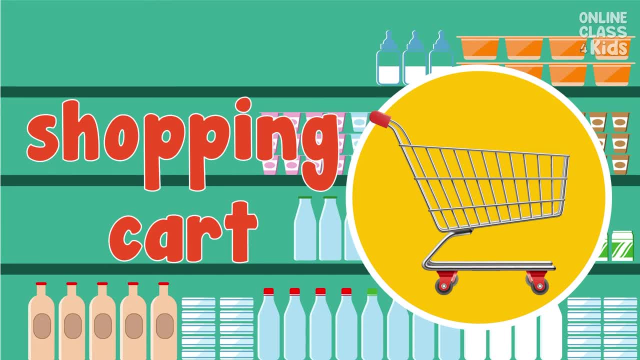 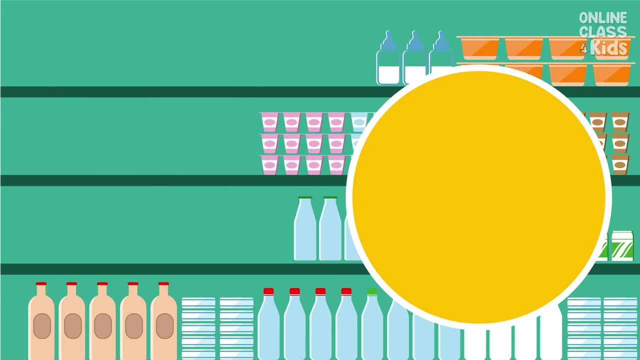 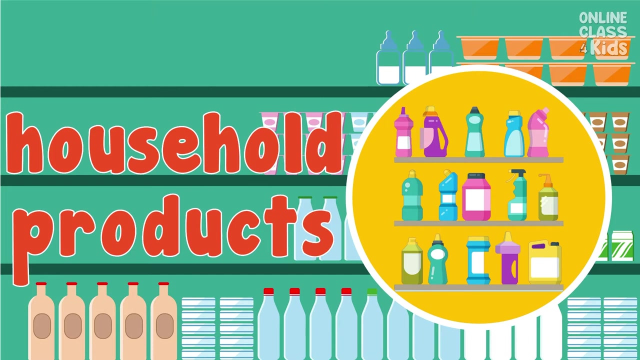 We need a shopping cart to put all the things we buy in the supermarket. It is a wheeled cart and sometimes appears small or big. Say shopping cart. First, I need to buy household products like shampoo, soap, dishwashing liquid and dust removers- Say household products. 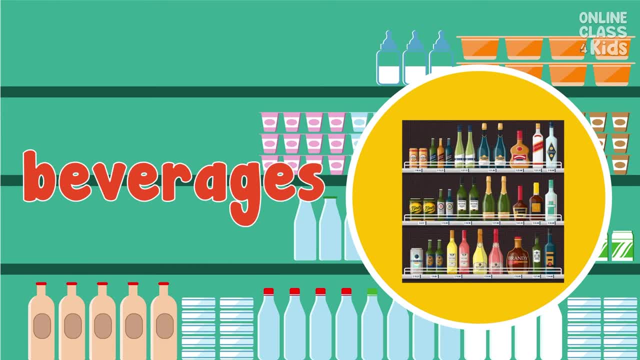 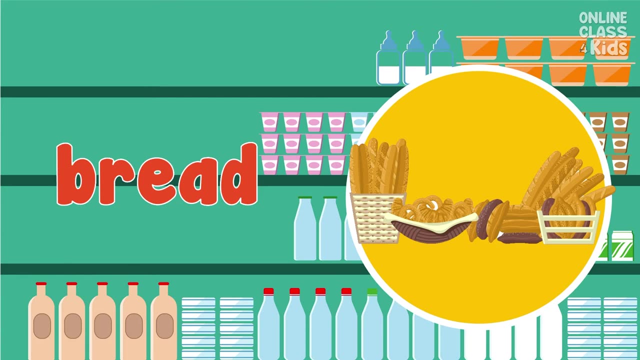 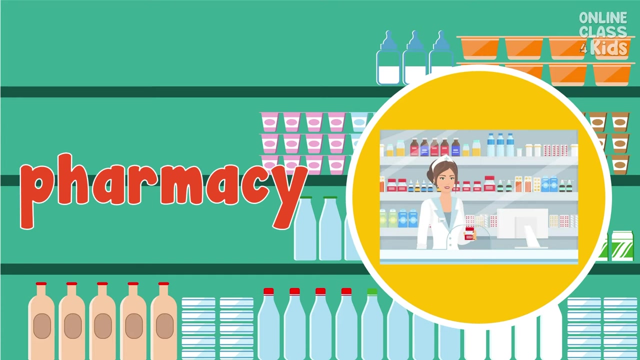 I love tea, Coffee or milk. I can buy these in the beverages- Say beverages. I like to eat bread for breakfast and I would love to bake too. Say bread. I need to drop by at this store later, where medicinal drugs are dispensed. 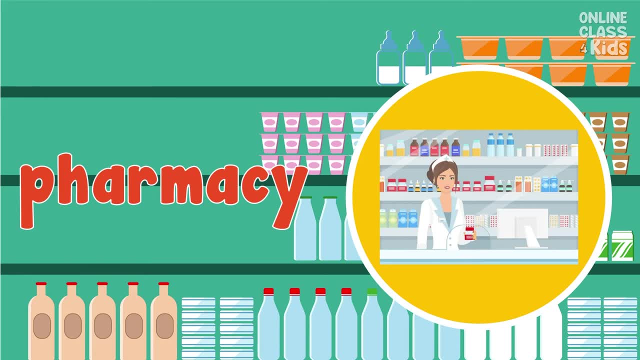 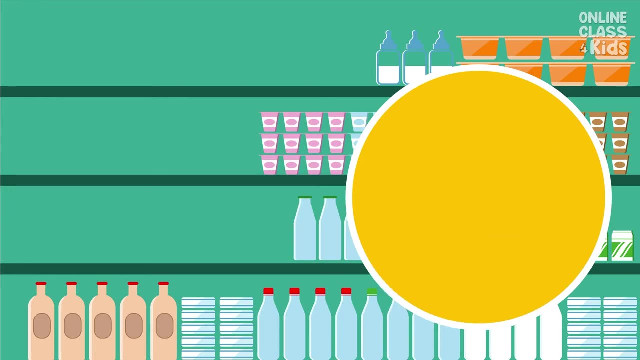 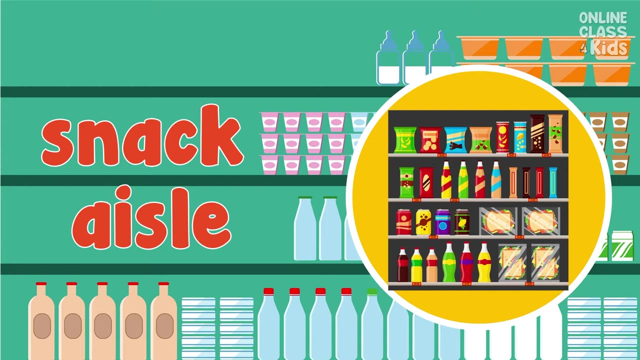 And so, in case somebody gets sick, Say pharmacy, Again pharmacy. There are no more potato chips and cookies at home. Let's go to the snack aisle. This is a place where you can find light meals or snacks. Say snack aisle. 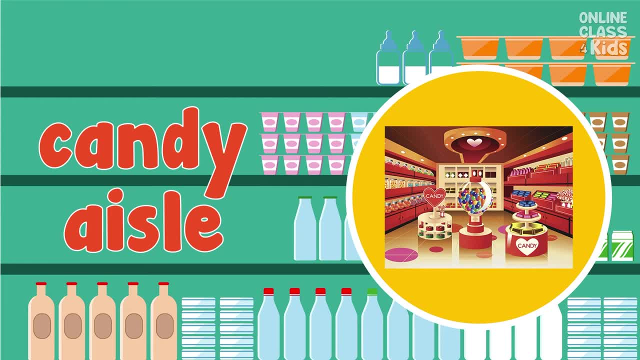 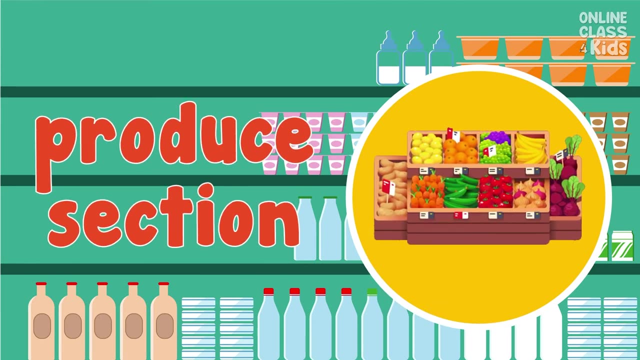 My sisters and brothers like chocolates, candy and other sweets. Let's move to the candy aisle- Say candy aisle. I'd like to buy freshly picked fruits and vegetables too. We can get these at the produce section- Say produce section. 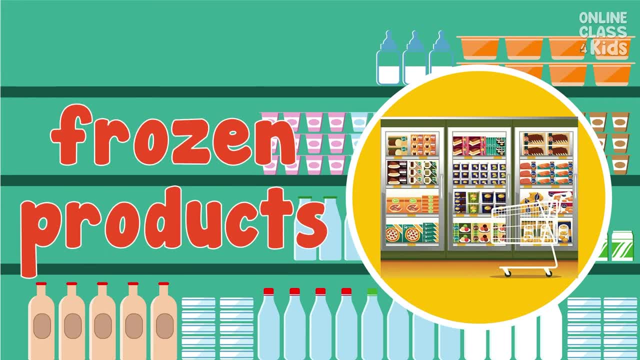 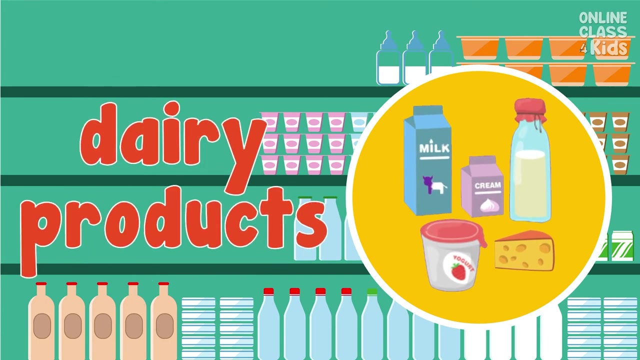 We love to eat pizza and steak for dinner, But not much time to cook. Luckily, we have these at the frozen products section. Say frozen products. It's healthy to drink at least a glass of milk in the morning and put butter on bread. I need to go to the dairy products. Say dairy products. 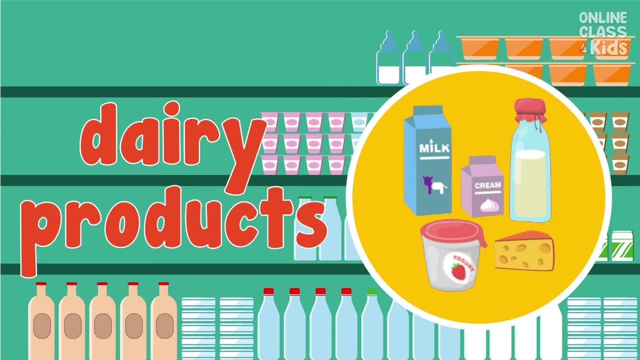 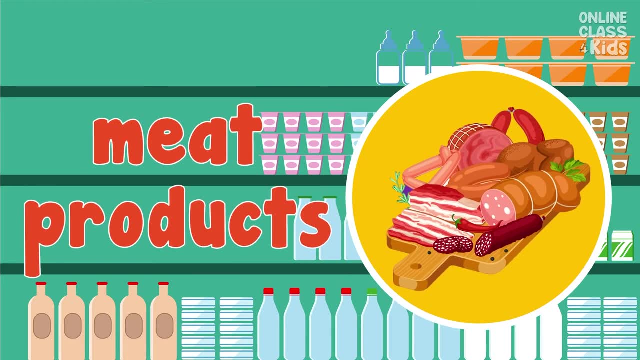 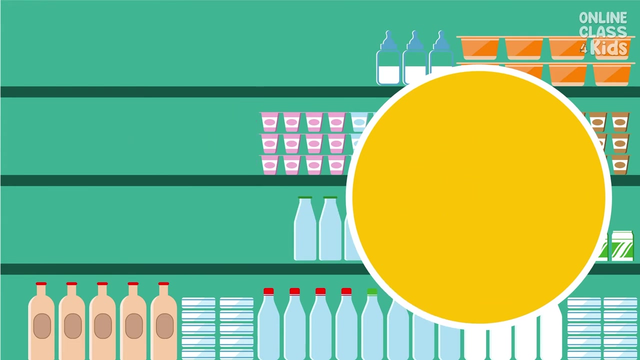 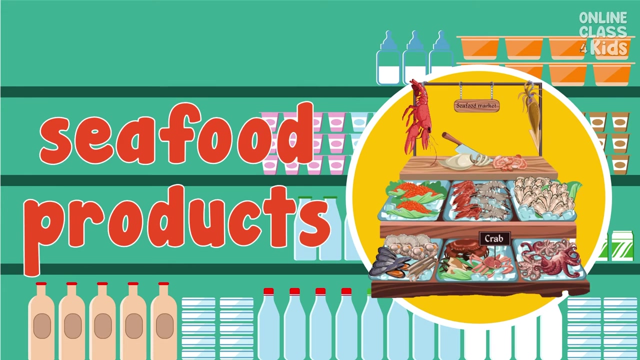 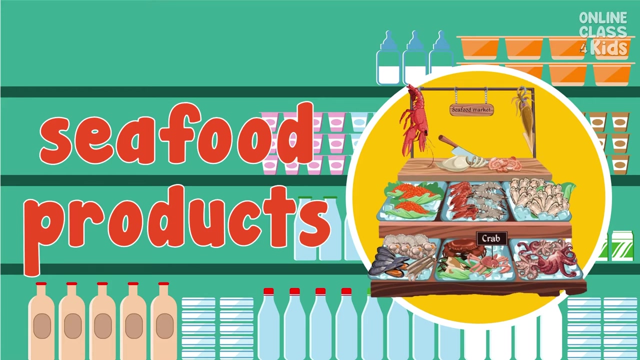 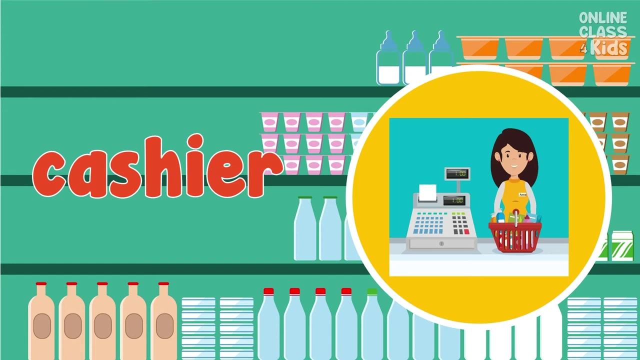 I just have some milk at home. I need to buy milk and butter- Say dairy products. We often have meat furniture too. We can buy beef gray bought in this store. just go to the seafood products- say seafood products. now it's time to pay. let's go to the nearest cashier. 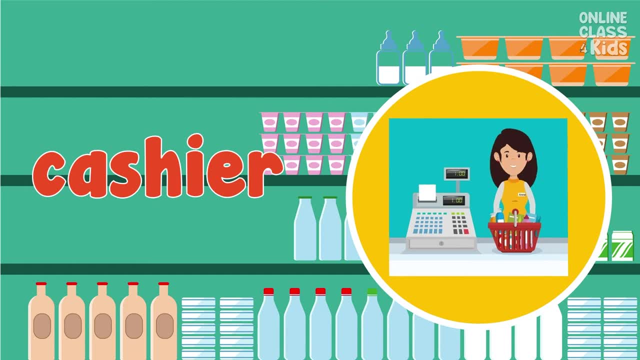 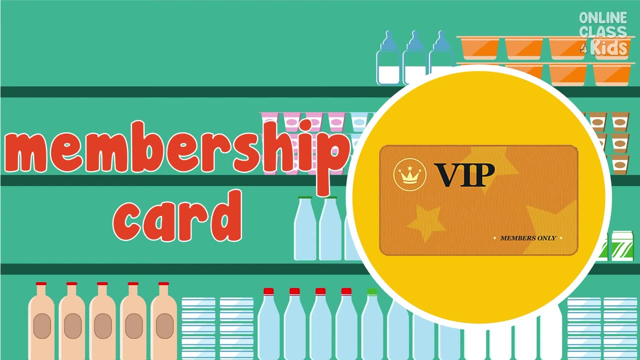 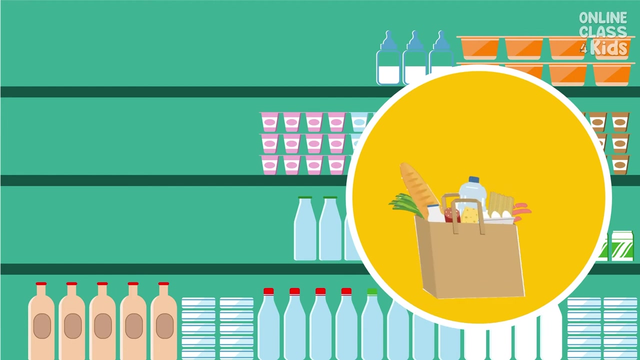 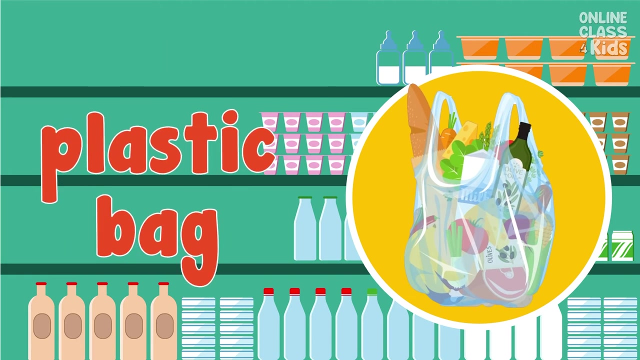 say cashier. mom often buys here, so she has a membership card. membership card is a small card issued to and held by a member of a club or organization. say membership card. we need a grocery bag to carry home our purchases. say grocery bag. it's okay to use plastic bag too, but make sure. 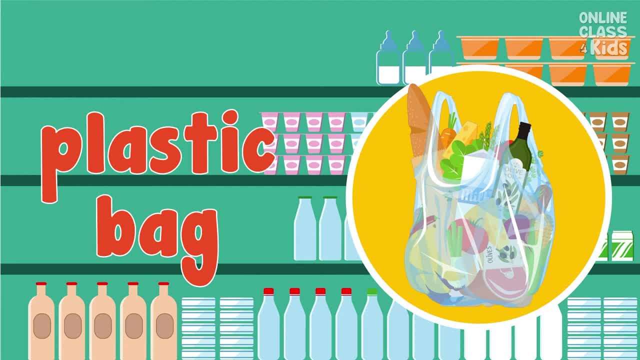 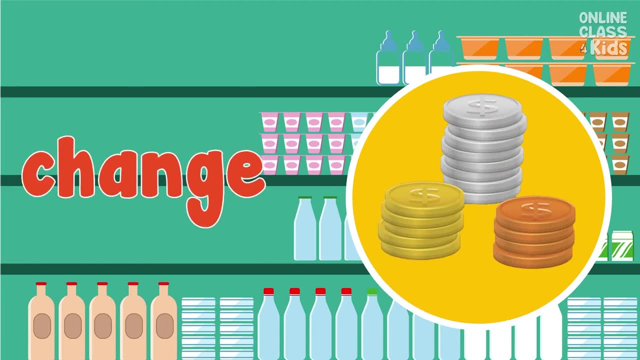 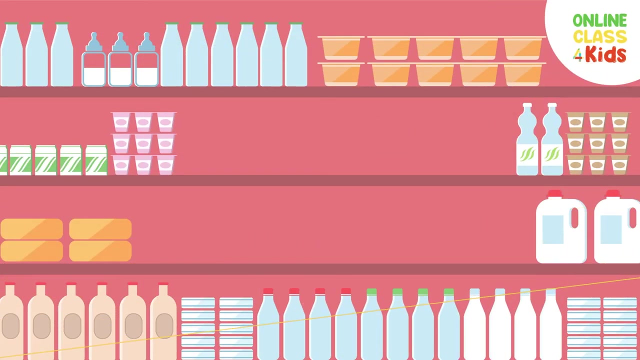 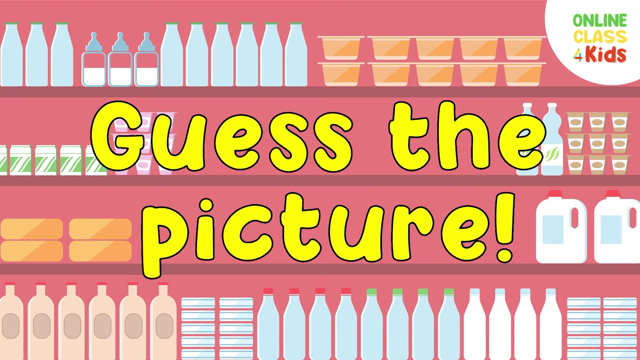 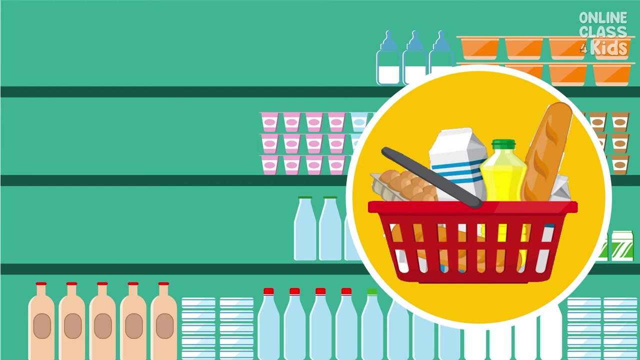 you recycle it. say, plastic bag. now i receive my change. this is the money given in smaller bills or coins in exchange for a larger bill, say change. let's review what we have found in the supermarket. help you guys taking pictures. can you guess these pictures? this is a shopping basket. 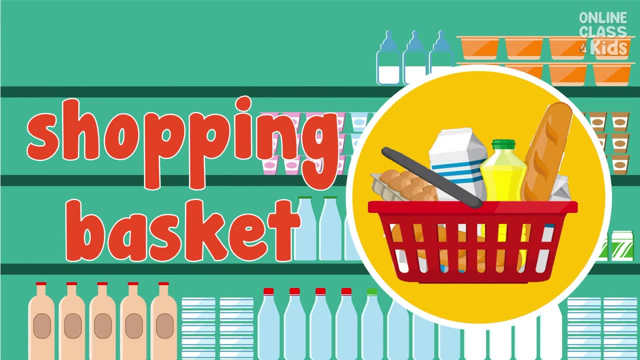 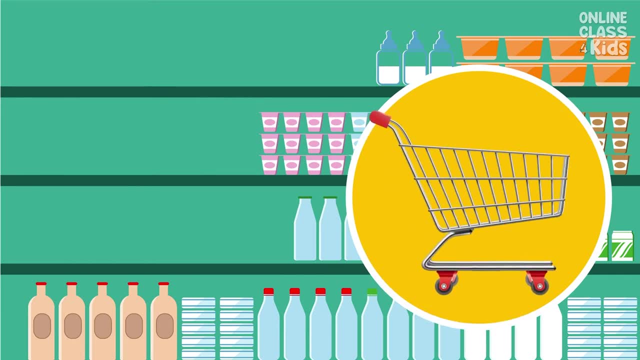 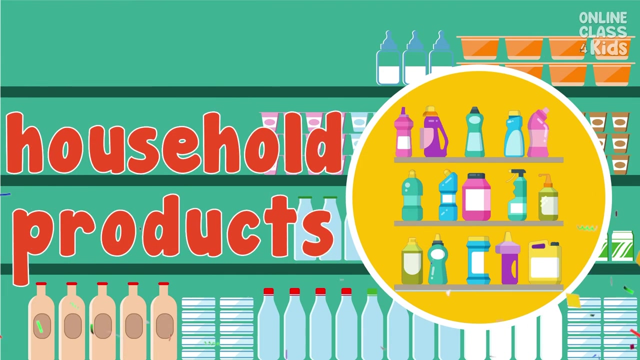 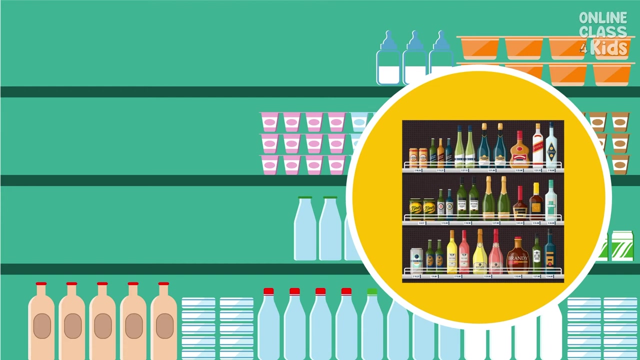 nice. a shopping basket, say shopping basket, shopping basket. can you guess what they say: shopping basket, shopping basket, shopping basket. Very good, It's a shopping cart, Say Shopping cart Nice. These are household products, Say Household products. You're right, Beverages, Say Beverages. 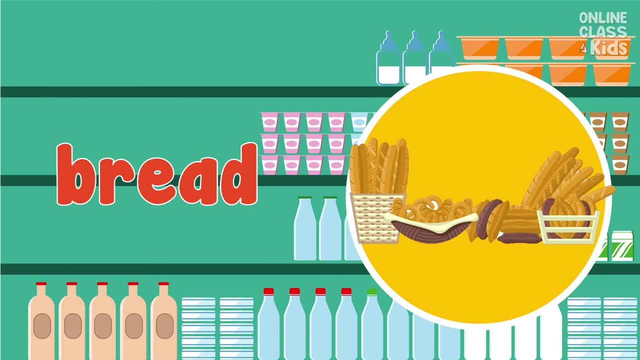 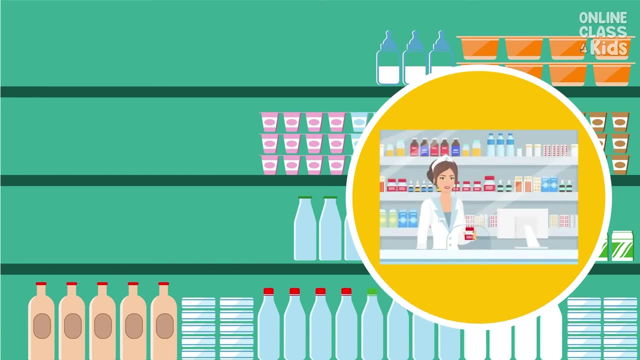 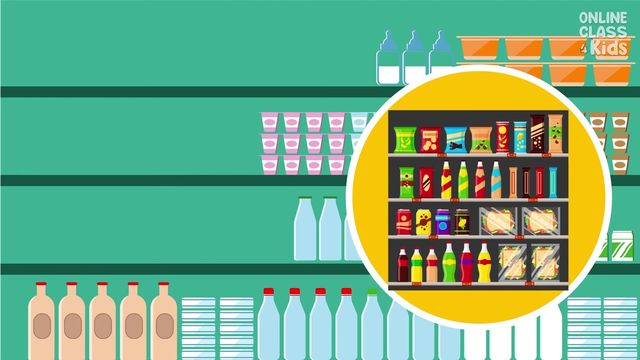 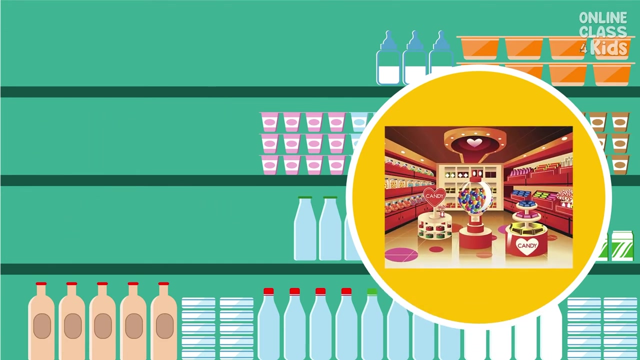 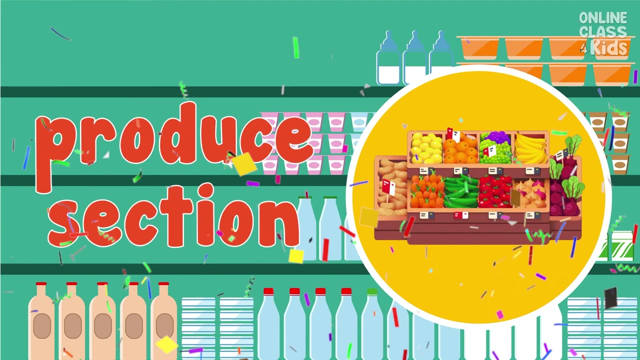 It's a bread, Say Bread. Very good, Pharmacy Say Pharmacy. You're right, Snack aisle Say Snack aisle. This is a candy aisle, Again candy aisle. Good job, Produce section, Again produce section. 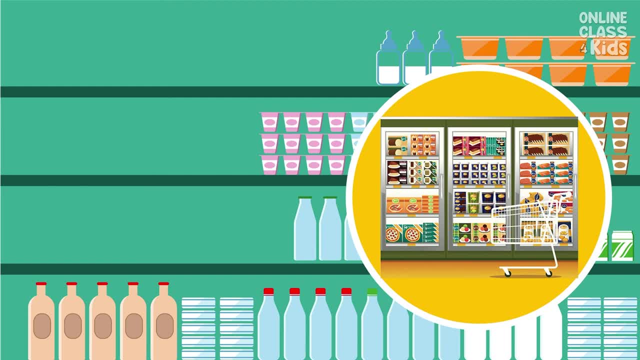 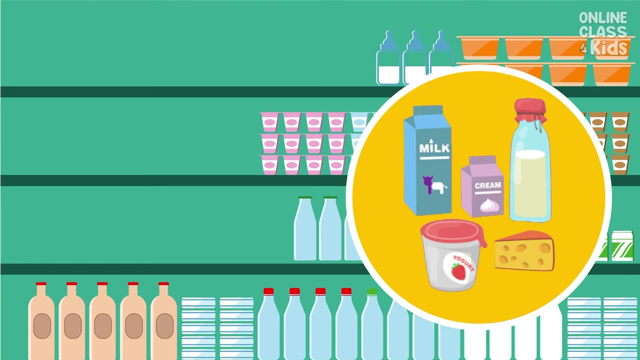 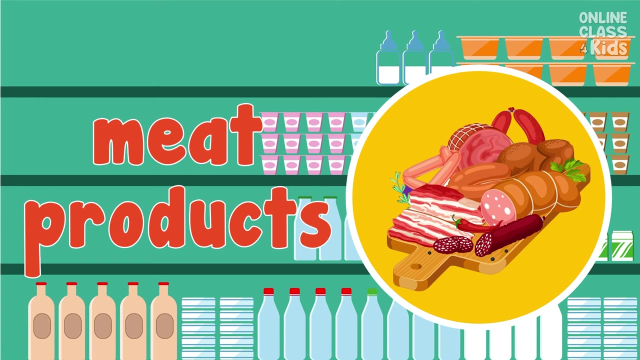 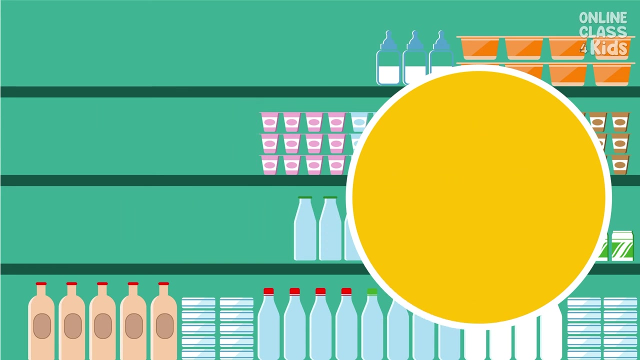 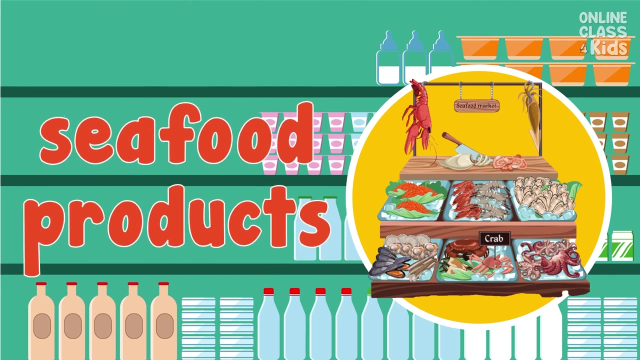 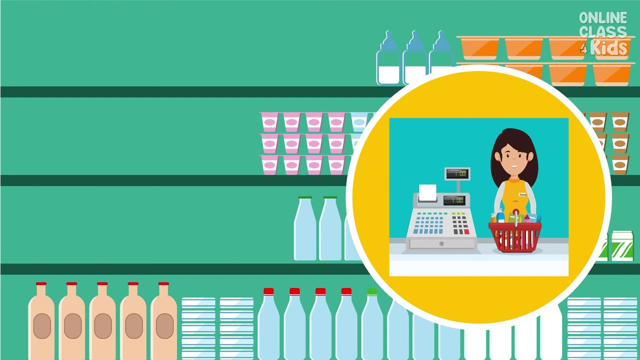 Very good. Frozen products, Again frozen products. Wonderful, Say Dairy products, Again dairy products. You're right, Meat products- One more time Meat products, Bingo. Seafood products, Say Seafood products. Good, It's a cashier, Say Cashier.